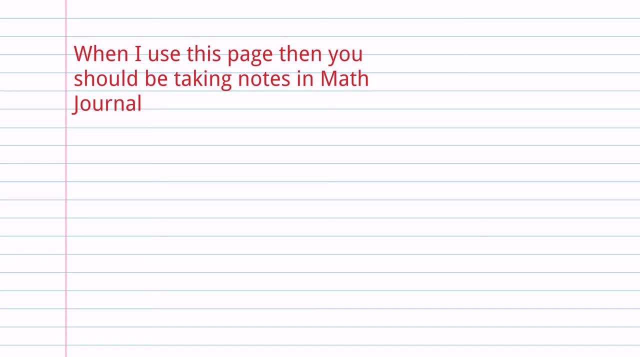 All right, let's go ahead and start off with a few tips or how we're going to do this. all right, So this is the I don't know. this is the binder sheet of paper background. So whenever you see this, this is when you need to be working in your math journal, the spiral notebook, the one that 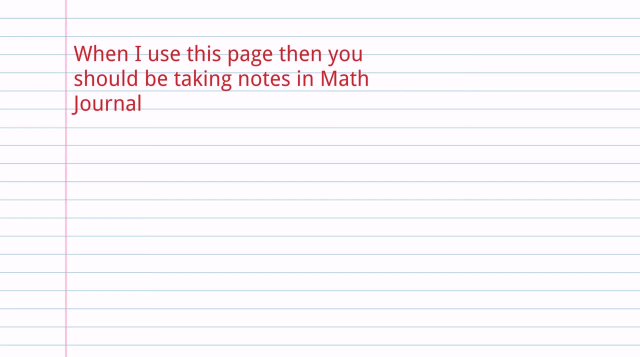 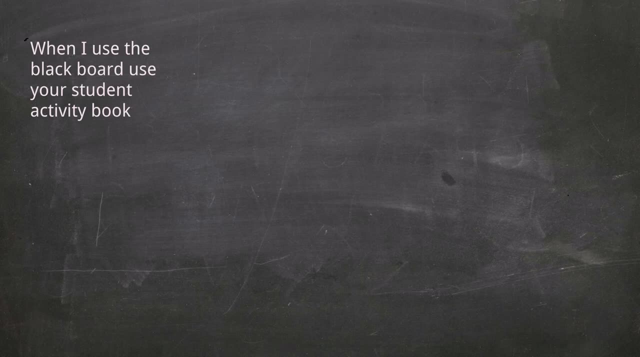 you take notes on. that's what you're going to be using this for. okay, When you see this background, the blackboard background, that's when you're going to use your student activity book. I'll take a problem out of there. I'll be working on problems in there. that's when you have to have. 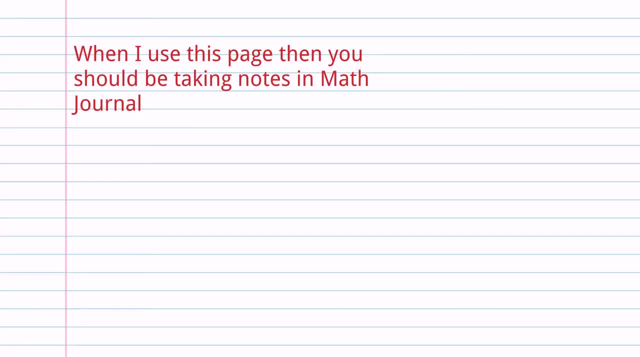 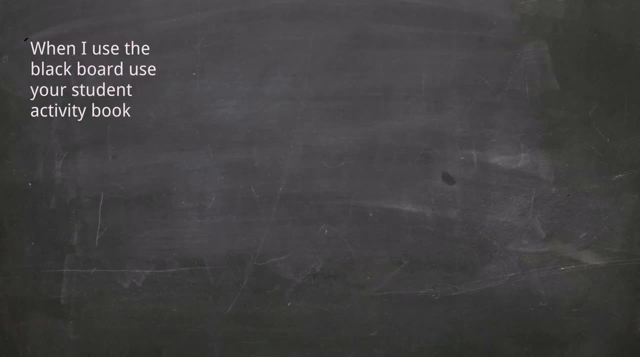 that out, okay. So when we use this, we're using our math journal. When we're using- when you see this, you're using your student activity book, Math journal, student activity book. all right, So let's go ahead and get started. I want you to go ahead and do. let's see here. I want you to 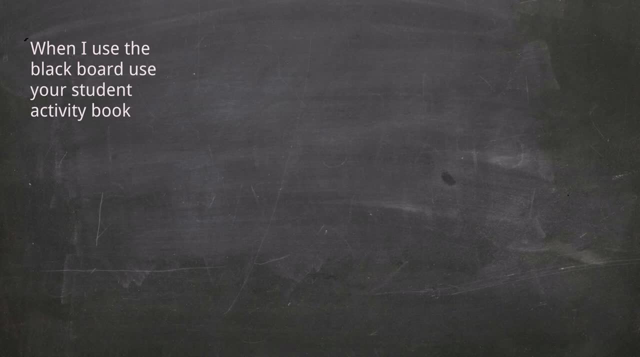 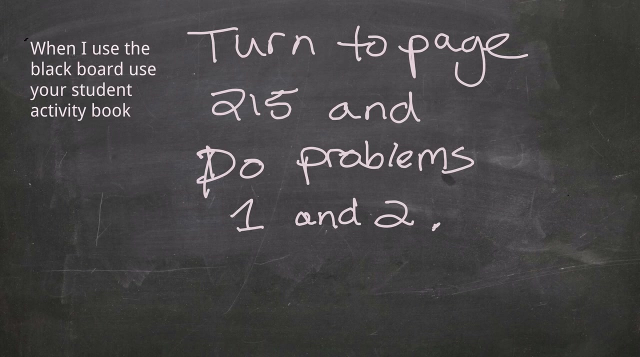 turn to page 215, and I'm going to see if I can write in here. oh, you can't see that and I don't like that. Let's pause it. Technology stop. All right, so I think I got it fixed. I want you to turn to page 215.. I want you to do problems. 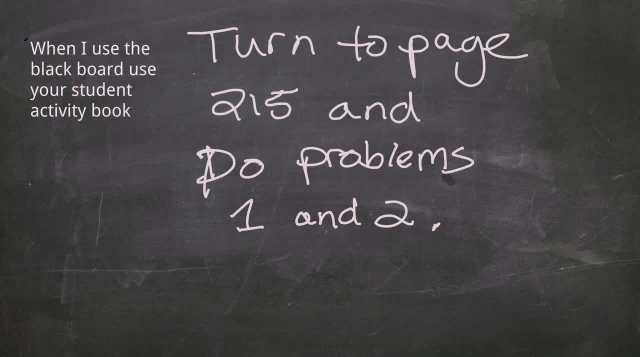 one and two on your own. That shouldn't take very long at all. I want you to do problems one and two on your own, So go ahead and do that first, and we're going to discuss how to solve that and we're going to talk. 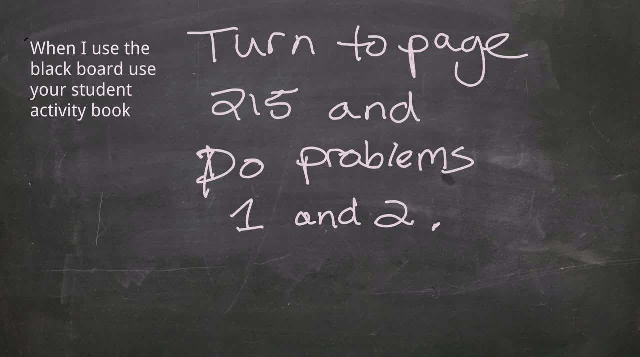 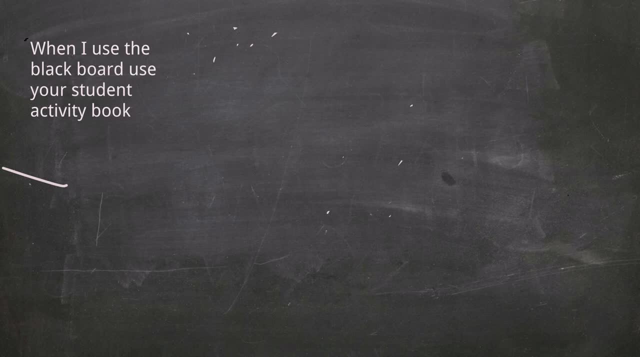 about comparison situations here today. all right, All right. so if we talk about questions one and two, they should have been easy for a reason, right? So number one, it used the word more, and then the number two: it used the word fewer. You've been doing word problems for a very 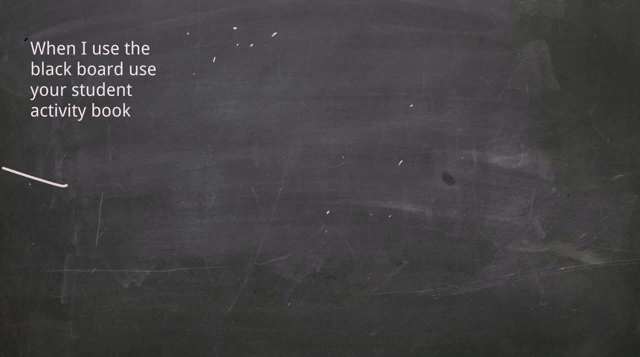 very long time. so if you hear the word more usually, it's an indicator, there's an addition or there's subtraction going on. When you hear fewer, well, actually, fewer is definitely a code for subtraction, right? So that's the reason why one. 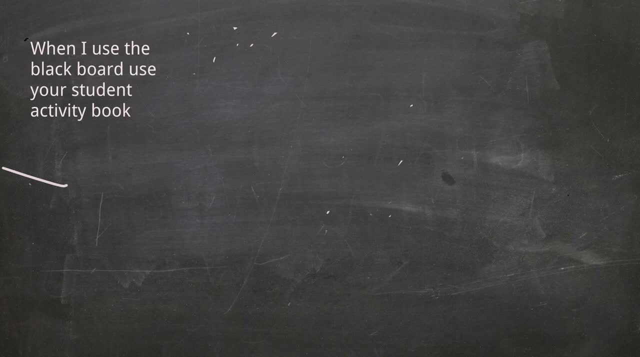 and two were fairly simple. So as we go further, we're going to like the other harder problems. the vocabulary is going to be a little bit different, so we're going to have to sketch those out. We're going to have to figure that out. We're going to slow it down. 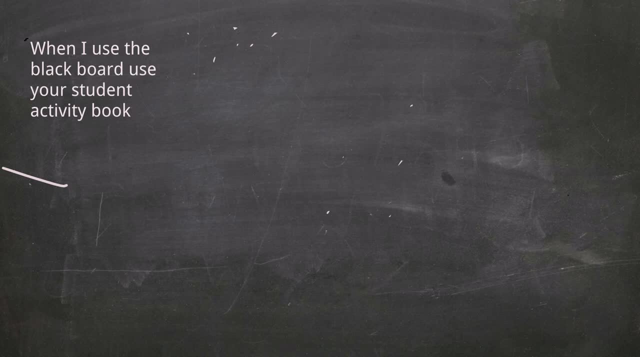 So with number three, let's go ahead and look at that. All right, so I went ahead and looked over the problems from one through seven here. We just did one and two right, And so I'm looking at number three. I'm just going to read it instead of typing. 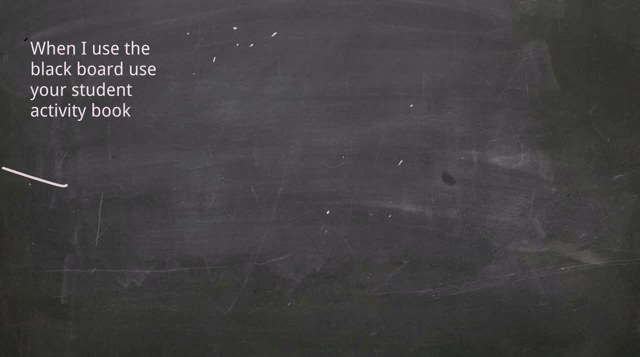 it here. It says altogether the jump, I'm sorry, altogether. the blue team jumped 11,485 times. The red team did 827 more jumps than the blue team. How many jumps did the red team do? So what are they asking there? They're asking: 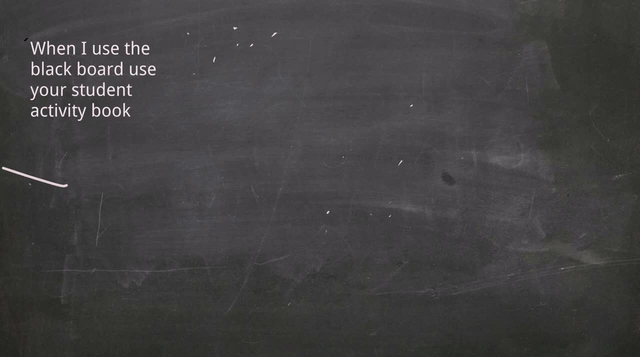 how many jumps did the red team do? So we're going to write down what we do know, So let me get that out. So we know that the blue did 11,485, right. And we know that the red team did 827 more than them, right. 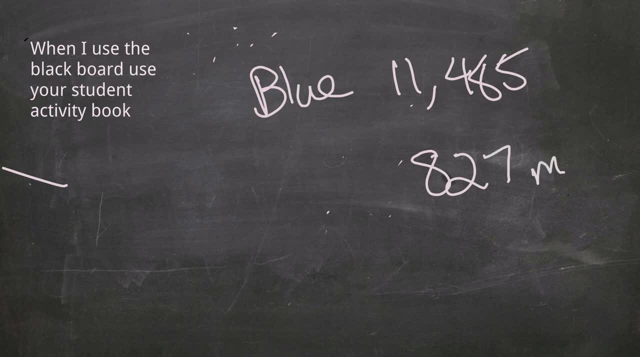 So 827 more red right. So if it's more, this right here should be whoops. I can't see that More is kind of the indicator that that is gonna be. what kind of problem? whoa, what is going on with this? 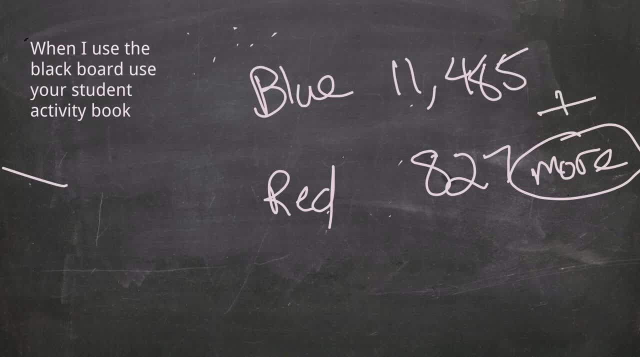 Okay, that is gonna be an addition problem, right? So you add it: five plus seven is 12, carry, whoops two and your answer should be 12,312,. all right, I'm gonna fast forward, I'm gonna go ahead and let you do four on your own. 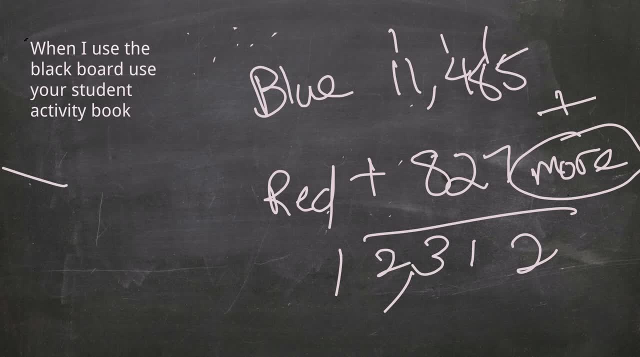 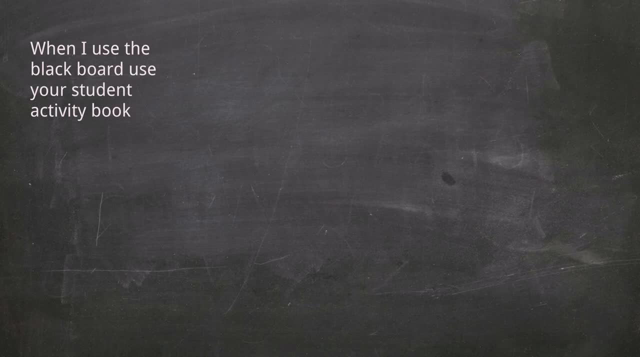 in just a second, but I'm going to clear all drawings. Yes, all right, and let's see here. I'm gonna skip to number five. It says Ted jumped 1300, or, I'm sorry, 1,300 times. 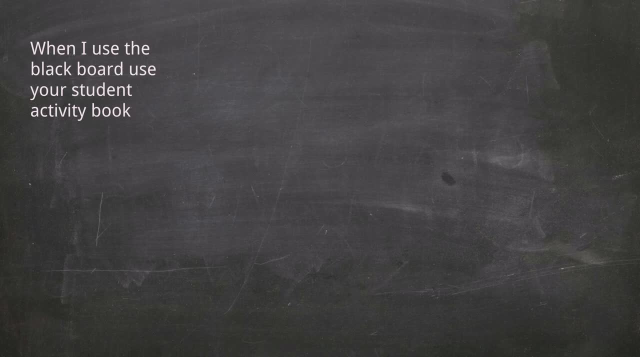 He did 100 more jumps than his friend Mario. How many jumps did Mario do? Well, let's go ahead and sketch that out, So I have my pen here. yeah, all right. So here is this. is gonna represent my good friend Ted. 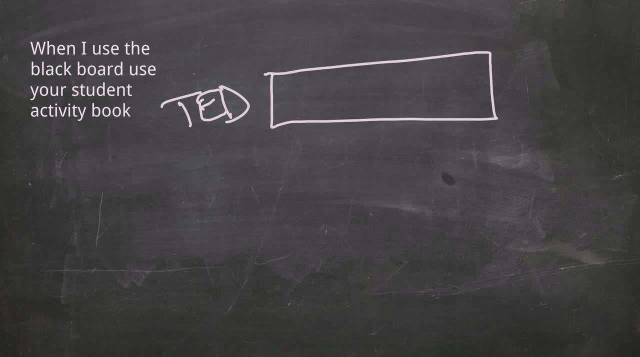 It's Ted, right, And Ted did how many? He did 1,000.. 1,300 jumps: He did 100 more than Mario. So here's Mario. Mario didn't do as much And Ted did 100 more than his friend Mario. 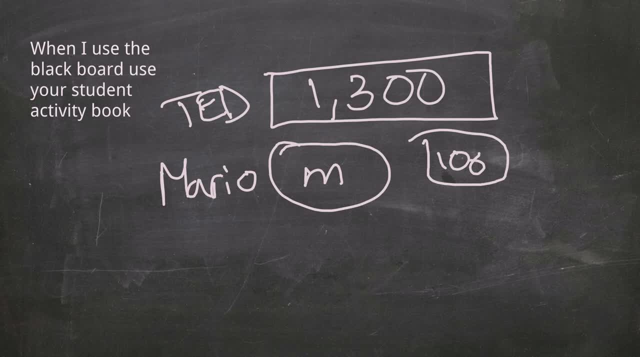 Mario did M. right, It's a variable. it's what we don't know, right? I know that looks like a six. I'm gonna change that. There you go, all right, So he has 1,300.. 1,300,. he did 100 more. 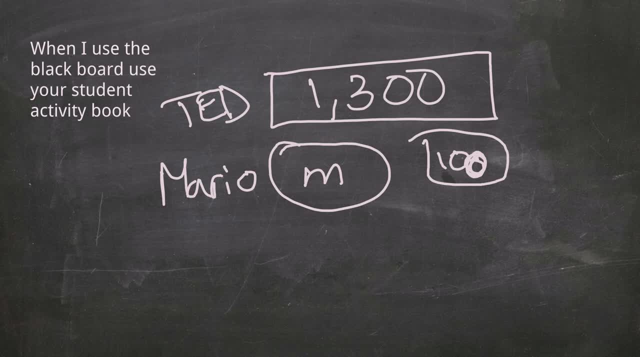 We have to figure out what Mario did. If you really think about it, M plus 100 should equal 1,300, right? Well, how do I figure that out? Well, the opposite of addition is subtraction. So 1,300 minus 100 should be or, I'm sorry. 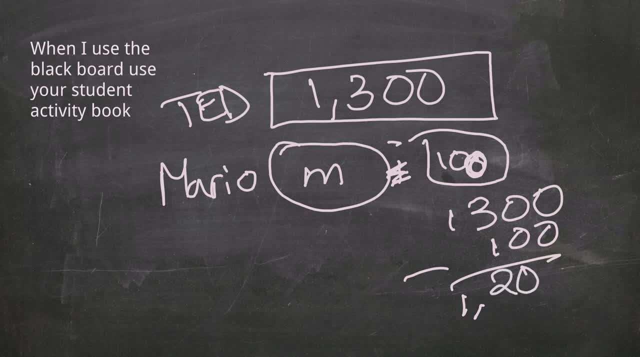 I say 1,300, it's 1,300, 1,200.. So let's double check our work. If we plug this in, 1,200 plus 100 should equal dun-da-da-dun, Ted. okay. 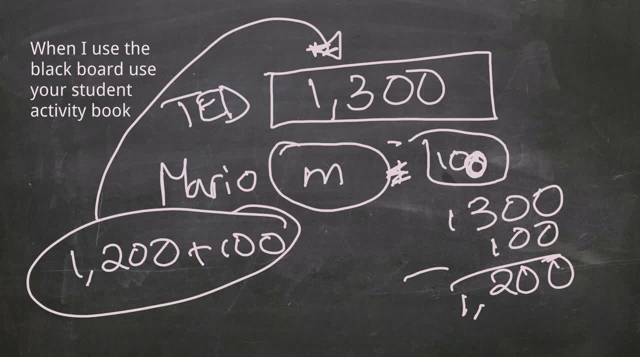 Do you guys see that? So sketching it out helps and I know this is a relatively simple problem, but if you get in the practice of sketching it out, it's gonna help you out a lot. all right, All right, in the interest of time. 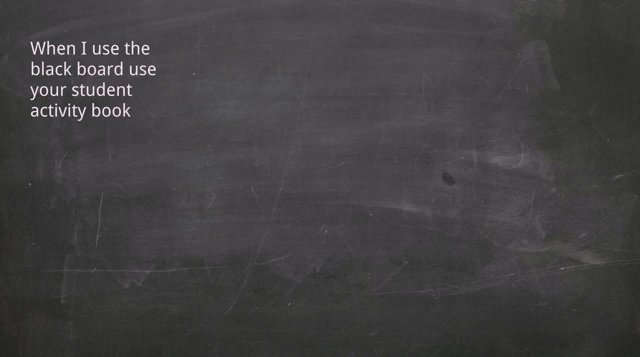 I'm going to skip down to number. actually, I'm not skipping down, I'm going to the next one, number six. Isaac jumped 900.. 987 times, 987 times. Who was that? That was Isaac. I'm gonna put Isaac here, all right. 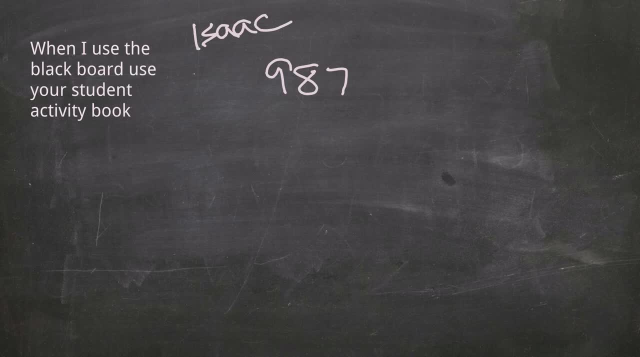 And Carlos needed to do 195 more jumps to tie with Isaac, right? So in order to tie with Isaac, he had to do 195 more. So who's behind, Isaac or Carlos? Carlos is yes, catch up. How many jumps has Carlos? 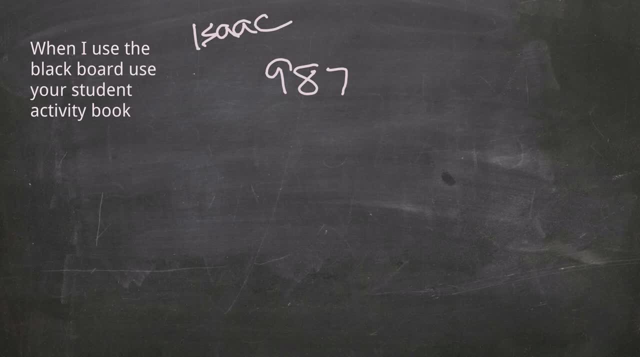 Carlos done so far. Okay, so let's think about that. This is how much Isaac has done, right, In order for Carlos to catch up, he needs to do how much? 195.. What we don't know, I'm sorry, let me write down Carlos. 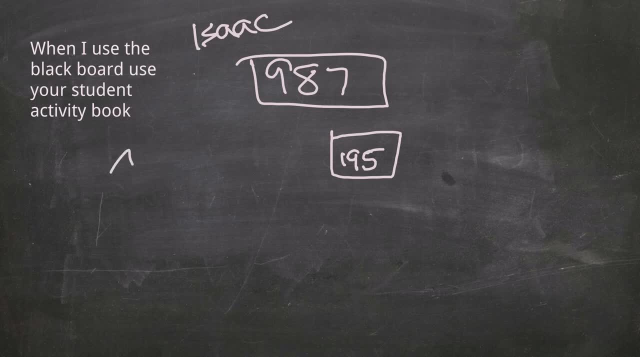 Is it Carlos? Yes, it's Carlos. Sorry, I'll get better at this, I promise All right, and so I'm going to put C as my variable, okay, So technically, our situation equation is: 987 equals Carlos plus 195.. 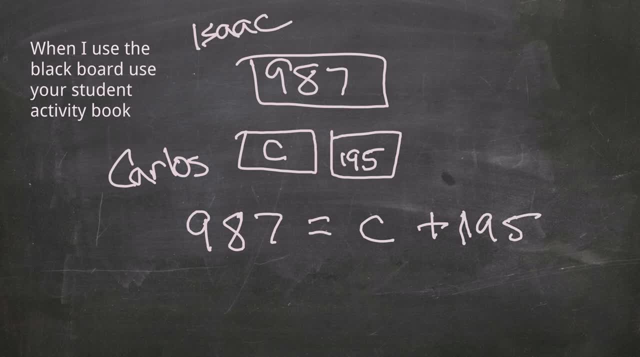 Now the question is: how many has he done so far? This is how much he has to do to catch up. This is how much more he has to do to catch up. This is what he has done. This is what they want to know. 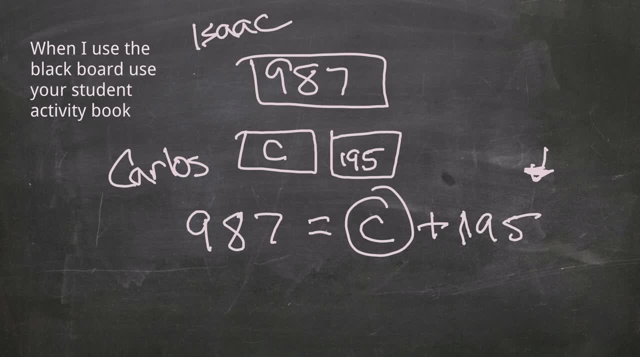 So the opposite of addition is: I should have heard subtraction. All right, so I'm just going to make it easy on myself here and I'm going to erase a few things here. Actually, I'm just going to put it underneath here. 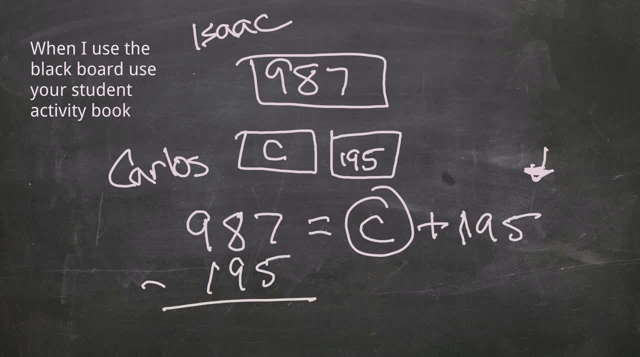 195 goes here. I subtract it: 7 minus 5 is 2.. Borrow here: This is 8.. This is 7.. This is 9.. Your answer should be 792.. Jumps, Don't forget your unit. 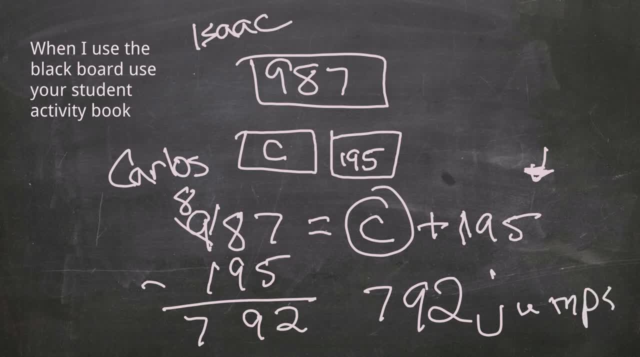 Whoops Jumps Ta-da, And for that you get a chicken. All right, I had too much fun with that. All right, now we are switching gears. I know there's a few more in there. I'm going to let you do those ones on your own. 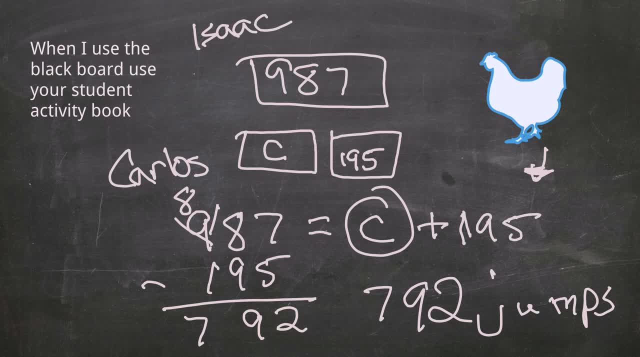 A lot of those, the comparing ones that we've done so far. those are addition or subtraction, all right, Or they're combining the two, depending on what you're looking at. I am going to clear all my drawings: Boom, clear. 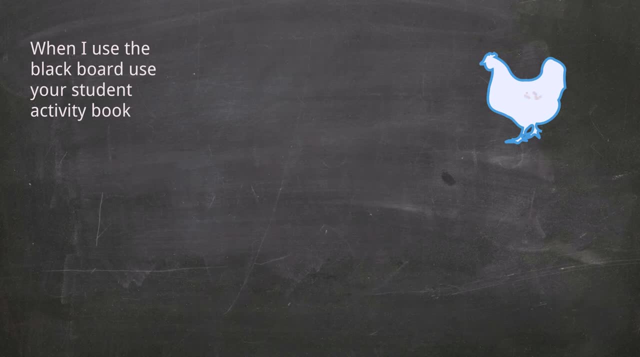 There it is. Oh, I'm going to get rid of this guy. I'm going to get rid of the chicken. I want to get rid of the chicken. All right, I'm going to pause. All right, let's go ahead and do number 8.. 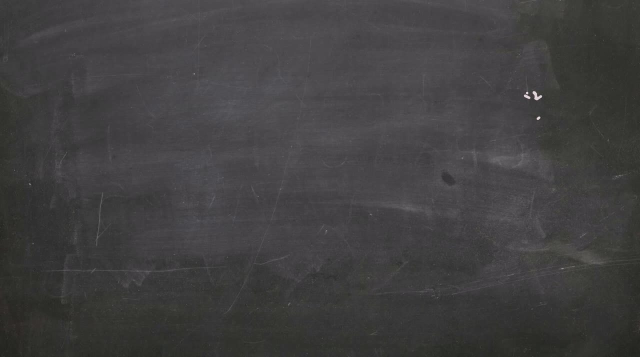 I want you to do number 8 on your own. It should be relatively simple. I'm going to read it real quick. Maria scored 6 points in the basketball game. Suzanne scored 4 times as many as Maria. How many points did Suzanne score? 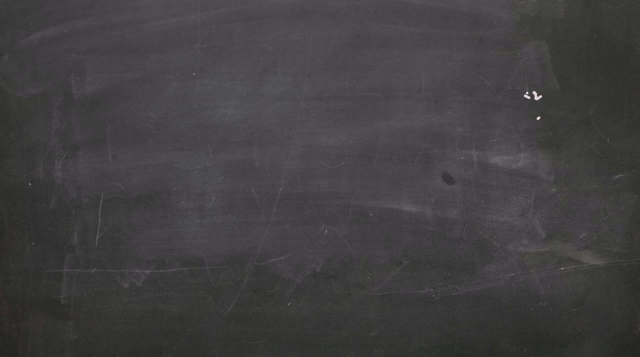 So we know that Maria, Maria, Maria, she had 6 points. all right, We know, Suzanne, Suzanne, how do you spell Suzanne? Suzanne, Suzanne scored 4 times what Maria scored. Well, what is that? She scored 6, 4 times 6.. 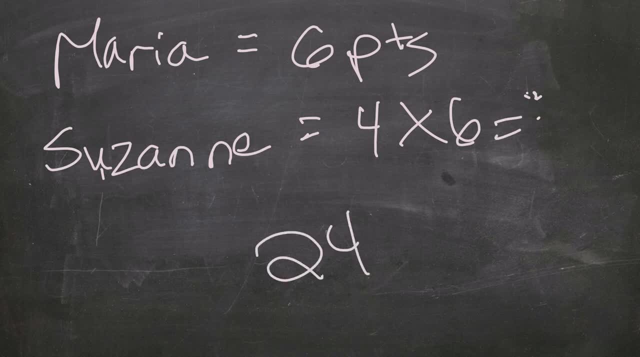 So 4 times 6, class is 24 points, And that's how you solve that. okay, So technically it's 4 times 6 equals. we'll do P for points and then, so P equals 24 points, all right? 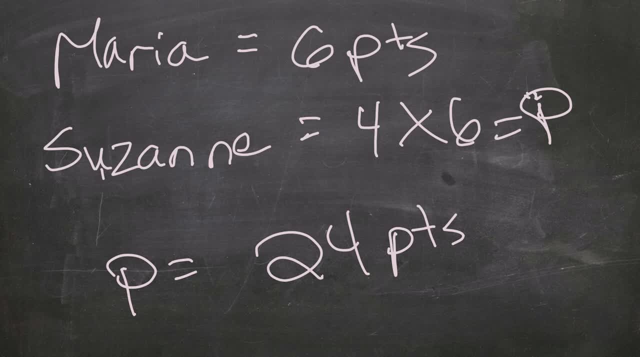 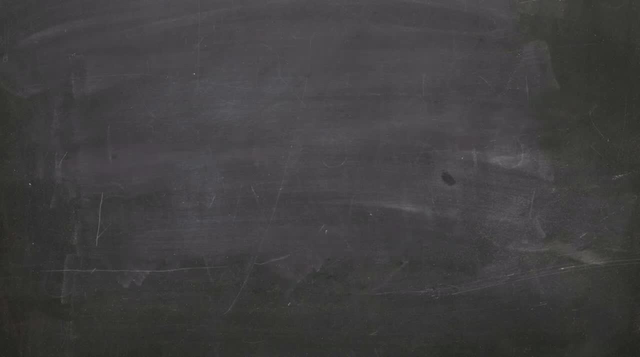 Let's go ahead and clear that. Clear it. Clear all images. Oops, clear, That's not it. Clear all drawings. There you go, All right, So let's do the next one. The next one is a little tricky. 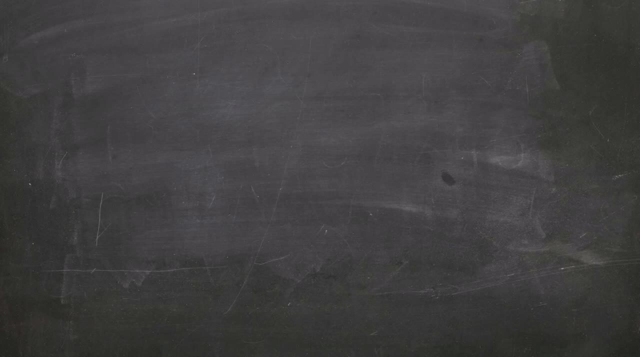 So Ramon scored 10 points at the volleyball game. I'm going to write that down because I need that information. Ramon equals 10 points. That was 5 times more as many as David scored. It was 5 times more than what David scored. 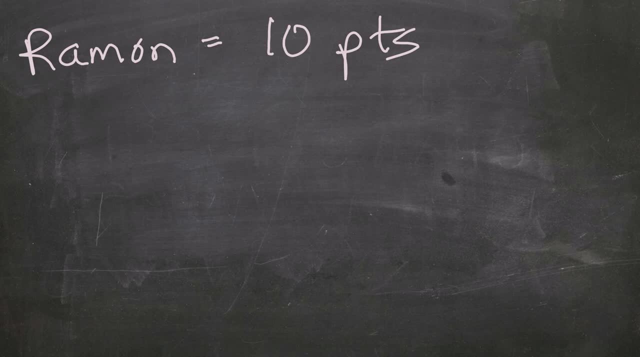 So do we know what David scored? No, we don't, all right. So we have D equals how much David scored. okay, Now we know that it was 5 times the amount that Ramon scored, right? I'm sorry, Ramon scored 5 times more, all right. 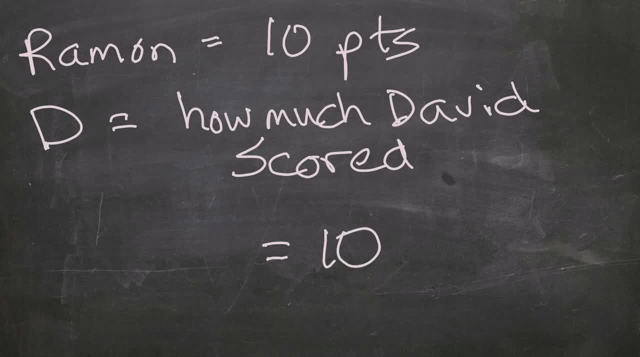 So if I have 10.. All right, I have D here and it was 5 times the amount because, remember Ramon, this represents Ramon. Whoops, I have a feature here. There you go. This represents what Ramon scored. 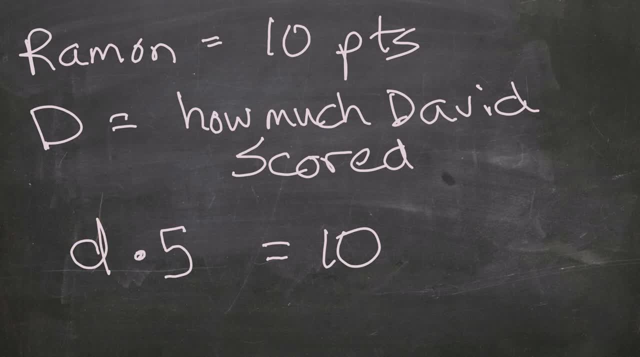 This is what represents what David scored. Who scored more? Ramon did, and he scored 5 times more. So David times 5 would equal Ramon. Okay, let's double. let's go over that one more time. David times 5 equals 10, because that's how much Ramon scored. 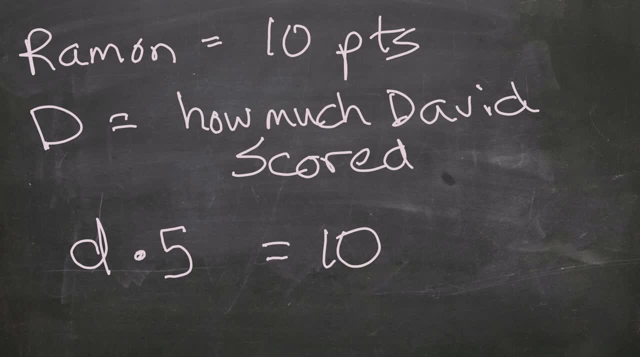 If I go back to the word problem, it says: Ramon scored 10 points at the volleyball game. That was 5 times as much, 5 times as many as what David scored. So plug it in there. what can go? there's only one number: D times 5 equals 10.. 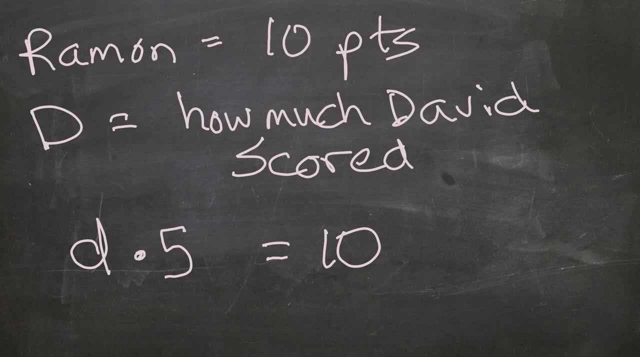 If I had to, we'll get that backwards. This is actually oops, let's see. yeah, there we go: 10 divided by 5, and my answer should be 2.. Sadly, David only scored 2 points. 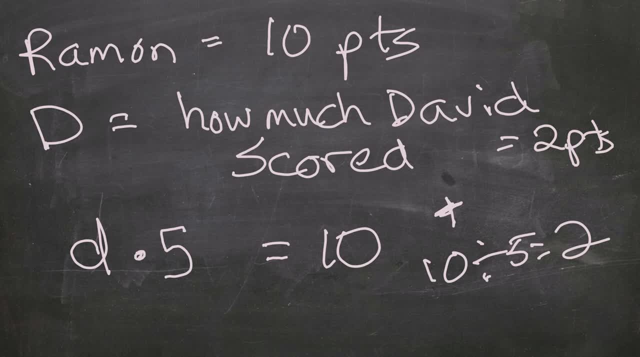 But if we plug it back in, is 2 point, I'm sorry, is 10 points, 5 times more than 2 points, Absolutely All right. and if I plug this back in here, 2 times 5 equals 10.. 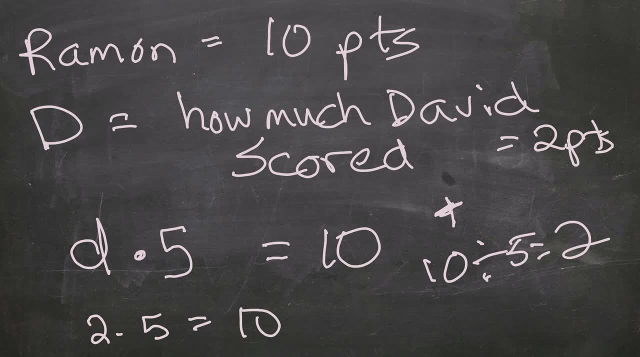 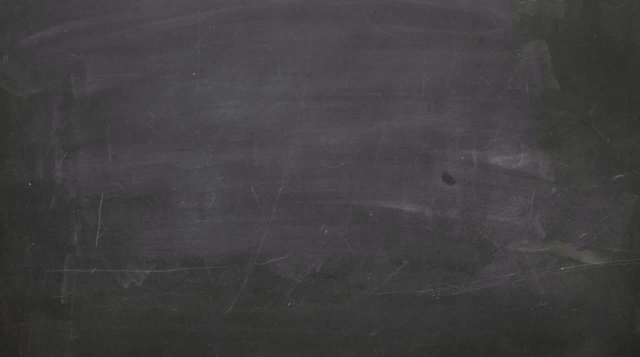 All right, All right, You know what I want to go back real quick, I just want to make sure I show you how to sketch these things. So if you wanted to sketch it out, here's Ramon. We said Ramon scored how many points. 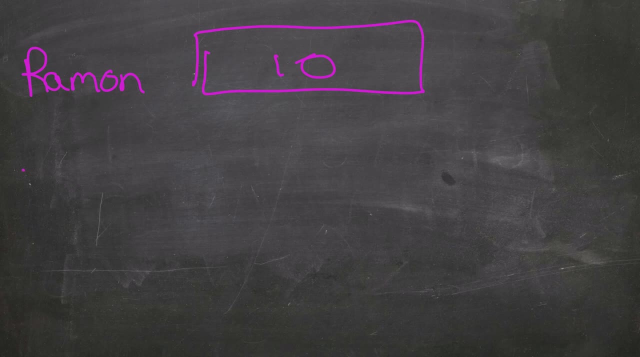 That's right, 10.. And we know that David, whoops, ah man, let's do this Eraser, All right. And then David, come on, David, all right, here we go. David, he did not score as much, right. 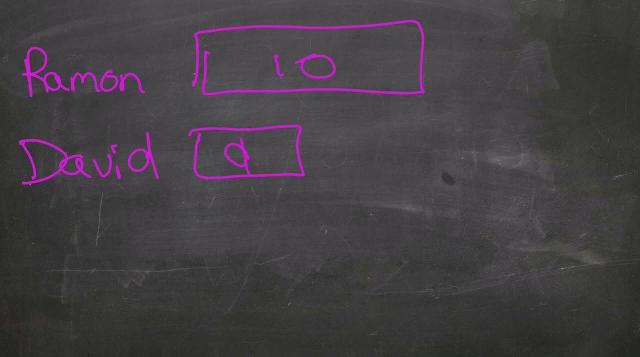 So D? okay, We do not know this part. Whoops, Is that right? Yeah, we don't know this part. No, I apologize, That's my bad. That's my bad, All right. So this is what we know. 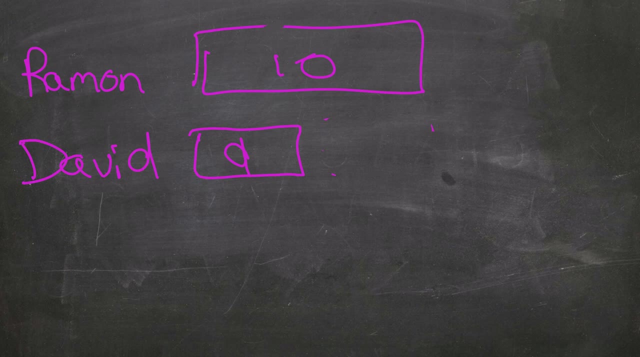 We know that Ramon also scored 5.. Oh my goodness, 5 times the amount of David, right? So, with that said, 5 times D equals 10.. Or you actually could do it this way, if you want: One fifth of 10 equals 2.. 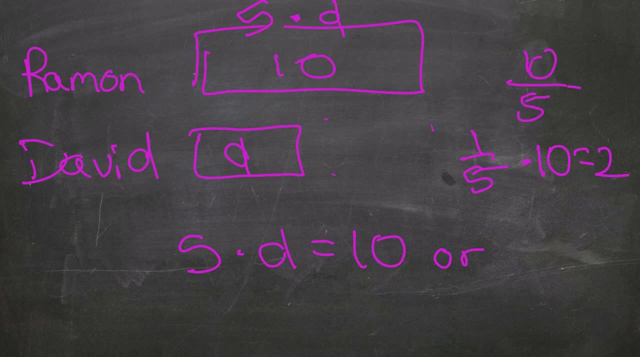 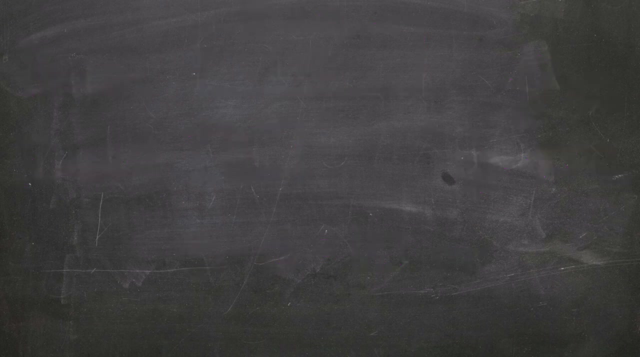 Because 10 over 5 equals 2.. All right, Boom. All right, I'm skipping down to number 13.. We're doing number 13 here. okay, I'll let you guys go back and you can work with a partner on the others. 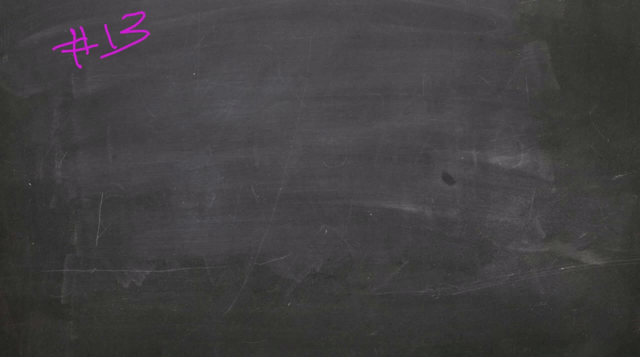 I just want to go over the more difficult ones here, All right, So I'm going to read it. Number 13. Chester has 49 CDs. Tony has one-seventh as many as Chester. All right, Just looking at that alone, who has less? 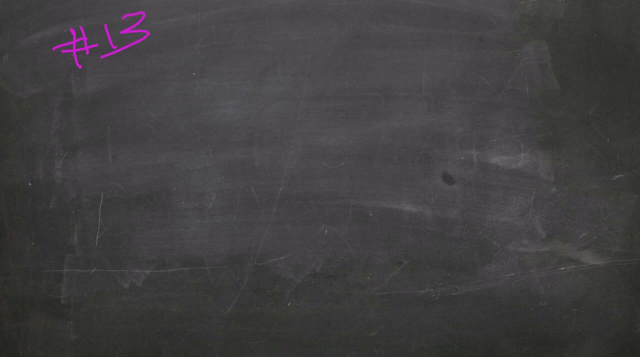 Chester or Tony. You should have said Tony. All right, Tony has less. He has one-seventh the amount. All right, How many CDs does Tony have? So if I'm going to sketch this out, I'm hoping you know that Chester had more. 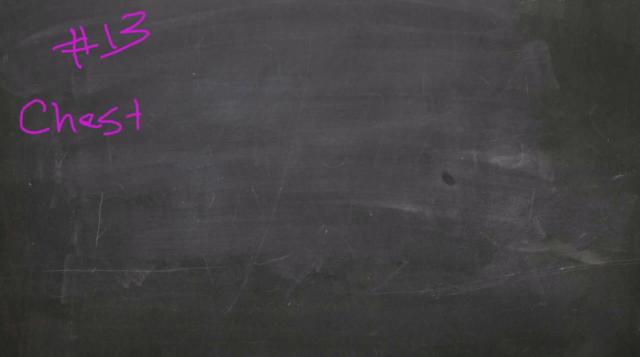 So, Chester, I'm going to put Chester here And I'm going to put Tony here. Now, Chester has more And he has 49 CDs. Okay, Tony doesn't have as many, Poor Tony, And if I look at it, he had one-seventh right. 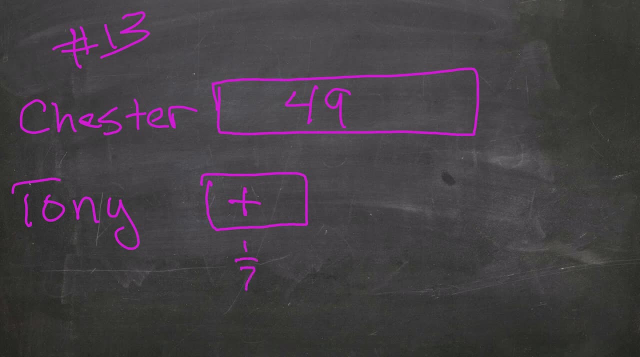 A T is going to stand for Tony, So he has one-seventh. All right, So he has one-seventh the amount of Chester. Or you can write that a different way. You could put: seven times what Tony has is what Chester has. 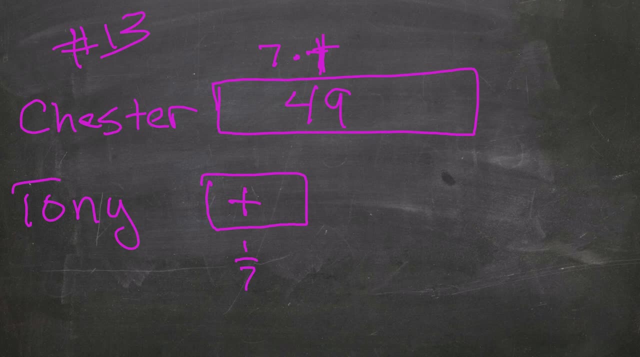 Right. So if I was going to make an equation, I could do two ways. I could go one-seventh times 49.. All right, 49 equals Tony, Or this is the way I like it. I like to do it: seven times T equals 49..